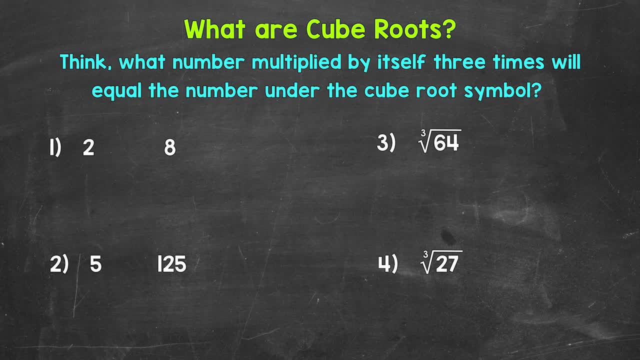 cube roots. we're going to start by looking at cubing a number, which means we have an exponent of 3.. For example, let's start with 2 cubed, so 2 with an exponent of 3.. This means 2 times 2 times 2, which equals 8.. So 2 cubed equals 8.. Again, 2 cubed, that means 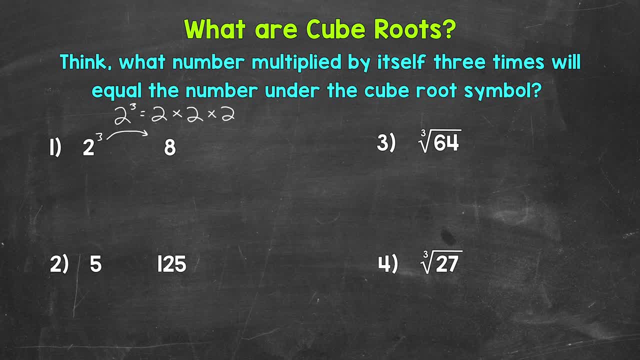 2 times 2 times 2.. 2 times 2 equals 4 times 2 equals 8.. Now, going off of 2 cubed, let's move on to looking at a cube root. Now a cube root is the. 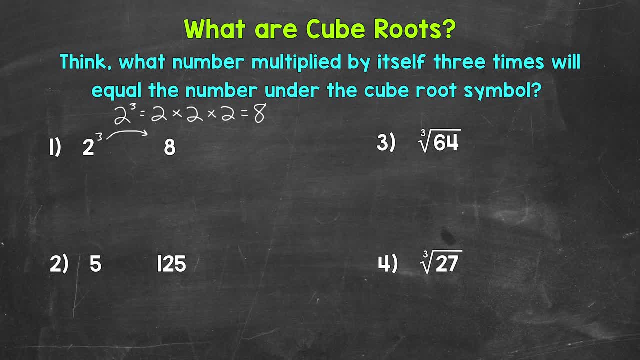 inverse of cubing a number, which means the opposite of cubing a number. We are going in reverse, so to speak. We need to think what number, multiplied by itself, 3 times, will equal the number under the cube root symbol. For example, let's find the cube root of 8. So 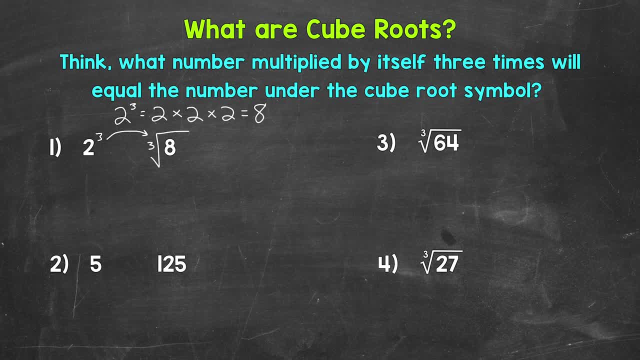 what number, multiplied by itself 3 times, will equal 8?? Well, 2.. The cube root of 8 is 2.. So again, the cube root of 8 equals 2.. So we can see the relationship there: 2 cubed equals 8,. 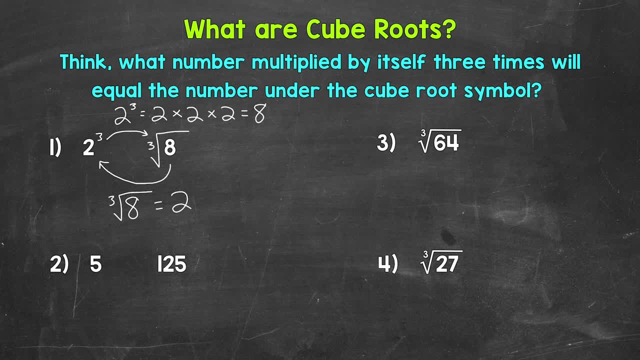 and then the cube root of 8 equals 2.. Let's move on to number 2 and take a look at another example. Let's take a look at another example. Let's take a look at another example. Let's take a look at another example. We have 5 and 125.. Let's start by cubing 5.. So 5 cubed and that. 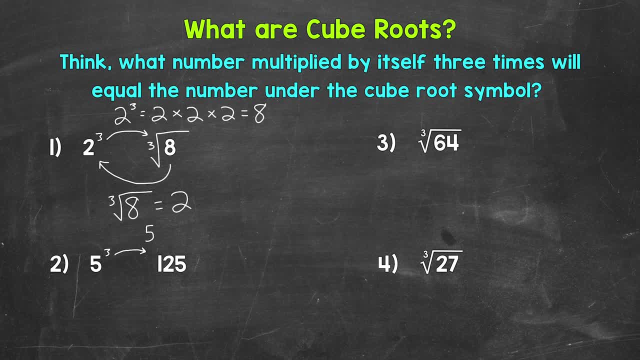 does equal 125. So 5 cubed that means 5 times 5 times 5, which again equals 125.. 5 times 5 equals 25 times 5, gives us that 125.. Now let's look at another example. Let's take a look at another. 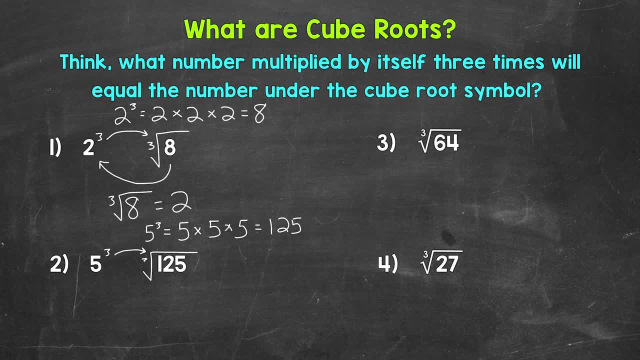 example, Let's find the cube root of 125.. So what number, multiplied by itself 3 times, will equal 125?? Well, 5.. 5 is the cube root of 125. So the cube root of 125 is 5.. So, to recap, number 2,. 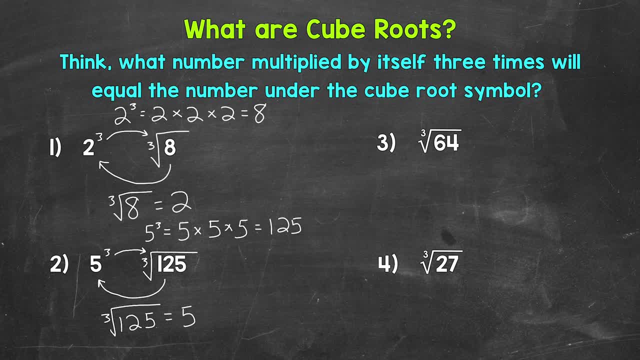 5 cubed equals 125.. 5 times 5 times 5.. The cube root of 125 is 5, because we know 5 multiplied by itself 3 times will equal that 125.. So we can see the relationship there between 5 cubed and the cube root of 125. 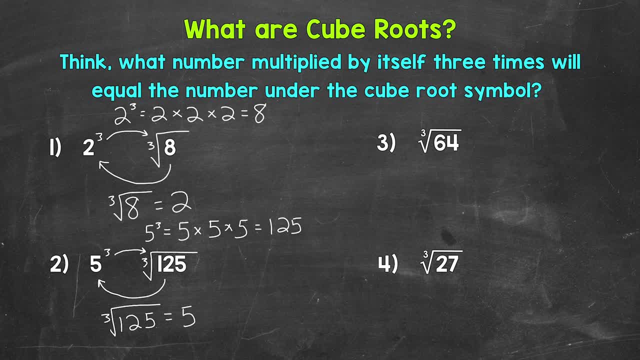 Let's move on to numbers 3 and 4, where we have two examples of cube roots, Starting with number 3, where we have the cube root of 65.. Let's take a look at another example. Let's take a look at another. 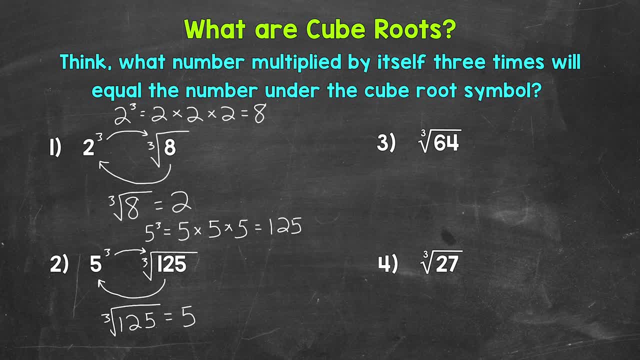 example, that's not complex. The cube root of 65 is the cube root of 64 times 64.. into 64.. So what number cubed will equal 64?? Well, 4.. 4 cubed equals 64.. 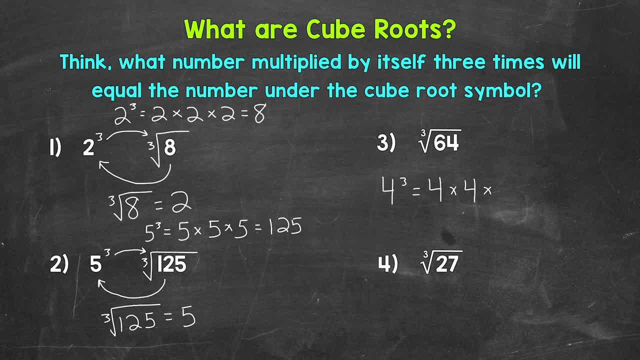 4 times 4, times 4.. 4 times 4 equals 16, times 4, equals 64. So the cube root of 64 is 4.. We need to think What number, multiplied by itself, three times a number of 64, is 64.. Well, let's keep looking. Sin number себе dances, Article S. If your peritoneum is чисоз, we need to figure out itshelpfulness. So now let's look at numberותic to removed numbers. If your peritoneum is чис, espero, what number multiplied by itself, 64 times 64, is 64.. 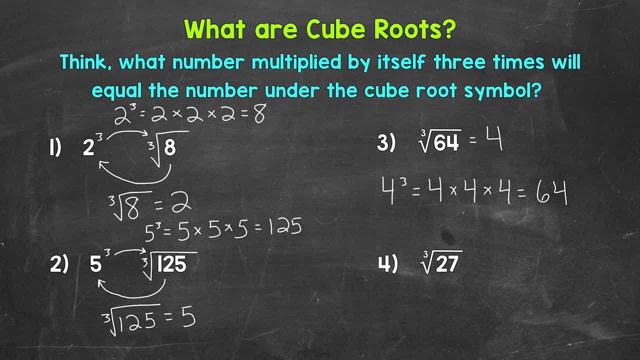 Well, the cube root of 64 is 4 times 64. So what number multiplied by itself, 3 times 4, equals 64? think What number multiplied by itself three times will equal the number under the cube root symbol. Lastly, let's move on to number four, where we have the cube root of 27.. So what cubed? 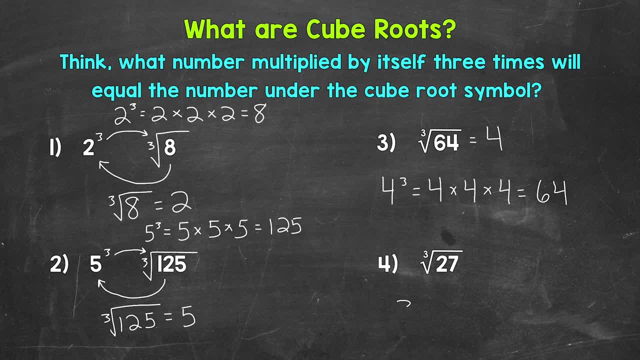 equals 27? Three Three cubed equals 27.. Three times three times three. Three times three equals nine times three equals 27.. So the cube root of 27 is three. So there you have it. There's a basic introduction to cube roots. Just remember what number, multiplied by itself three times, will equal.